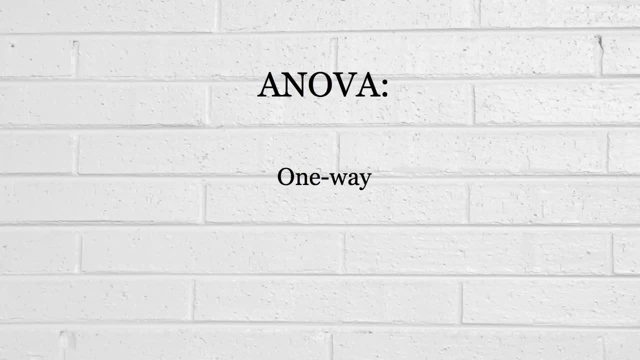 previously dealt with that topic, But here we're actually dealing with it in a more pure form. We're dealing with it as it applies to a single variable, and this is what we call one-way ANOVA. If you're keen on seeing how ANOVA applies to regression, I'll put up a link right here. 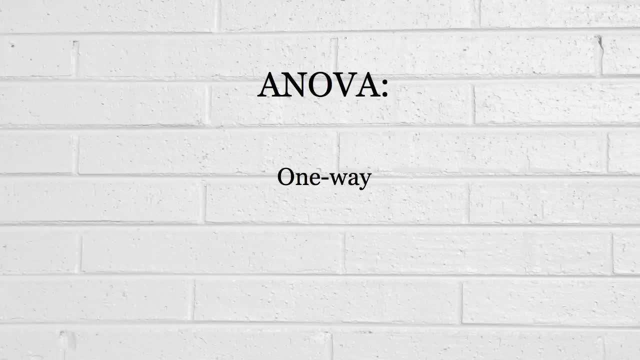 that you can follow to my series of regression videos, and this will be the one that will deal with ANOVA as it applies to regression. Let's get on with ANOVA in a one-way context. So first step is to consider what variance actually is. Now, hopefully you've. 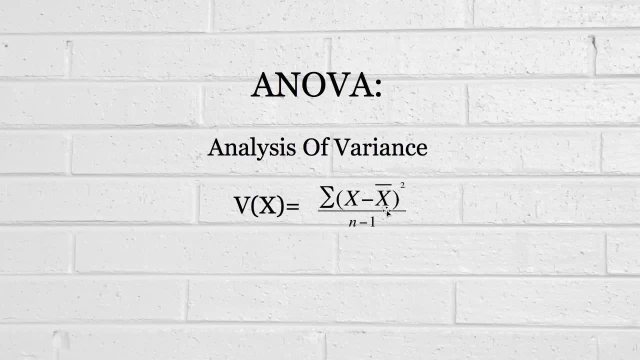 seen this formula before, but if we look at it, it's just the deviation from the mean of each observation. observation x. we calculate its deviation from the mean minus x bar, and then we square it and add them all together. that's what that sum symbol means, and so we're essentially finding some. 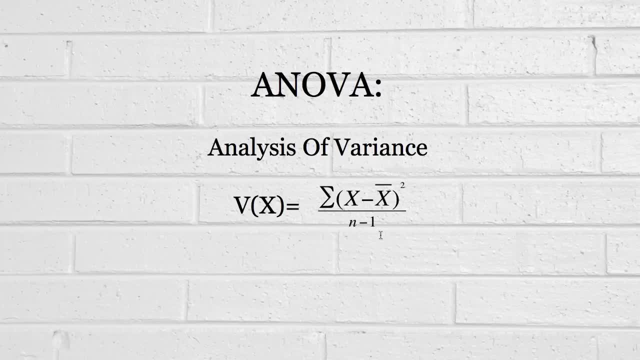 measure of the spread of the data. now, don't worry too much about the n minus 1 for the moment, because realistically we're only at this stage interested in that numerator, the sum of squares, which we're going to call SST, or total sum of squares, sum of squares, total. so in a sense you 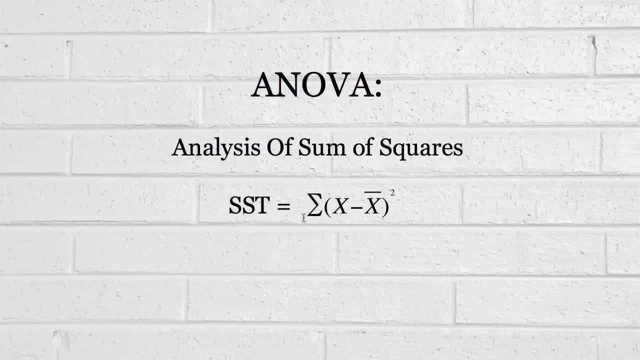 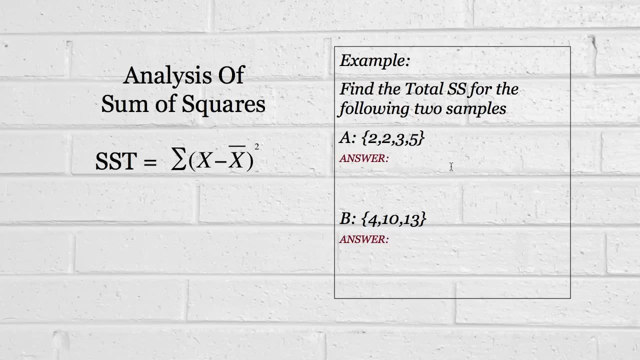 can call it the analysis of sum of squares as opposed to the analysis of variance. so, as an exercise, I'm going to get you to try and find the total sum of squares for the following two samples here's: a and b, and what I want you to do is try to use this formula here and find that. 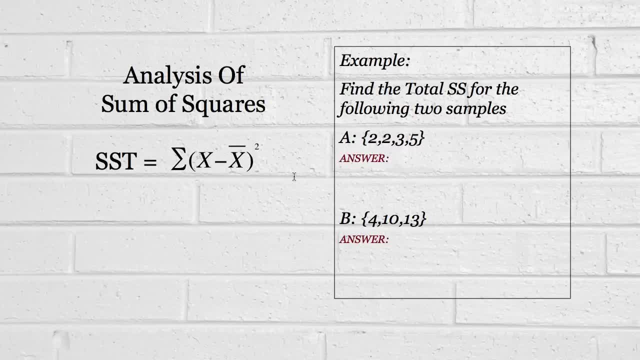 figure the SST for both of these and I'm going to get you to try and find the total sum of squares for both of these two samples. it's really quite crucial to get your head around what SST represents, so I'd recommend pausing the video and seeing if you can come up with the answers. 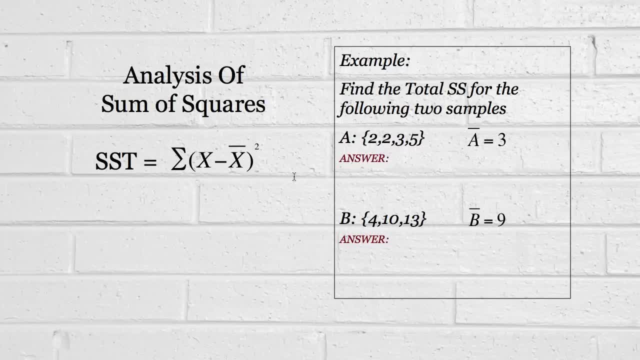 so, with that done, the first step is to find the means of these two samples, which is simple enough. the mean of a is three and the mean of b is nine. now the SST for a, using this formula. I'll just go through it very, very quickly. we take each of these observations in turn. 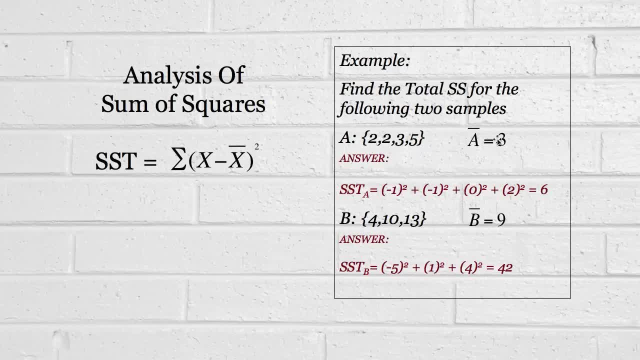 so we go two and then we subtract three, we subtract the mean, and then square it. two minus three is minus one, and we square it two again. minus three is minus one, and we square it, etc. and then we get a sum of squared total or total sum of squares of six. and if you tried it with b, 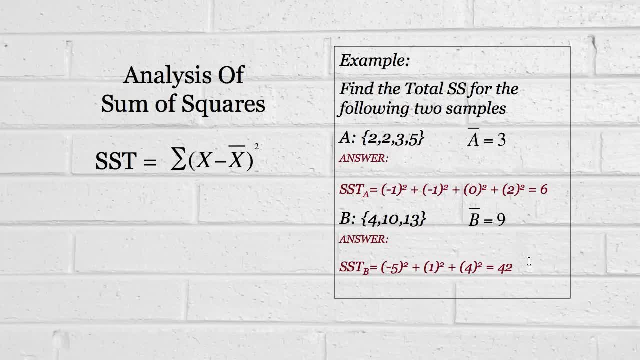 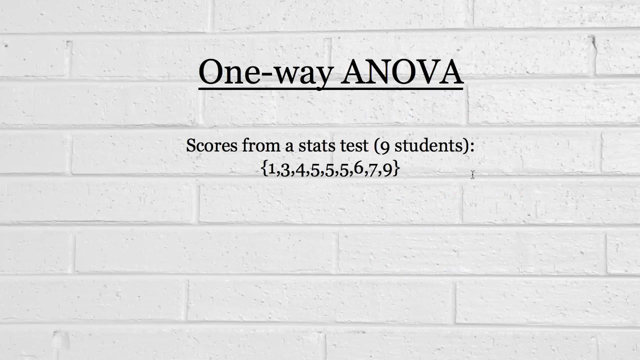 you should have got 42 and you can see that the larger the SST, the greater the spread of the data, and that's evident. look at a and b respectively. b clearly has a higher spread or variance, and that comes out in the sst. let's not forget, this is the numerator of the variance equation anyway. so let's have a look. 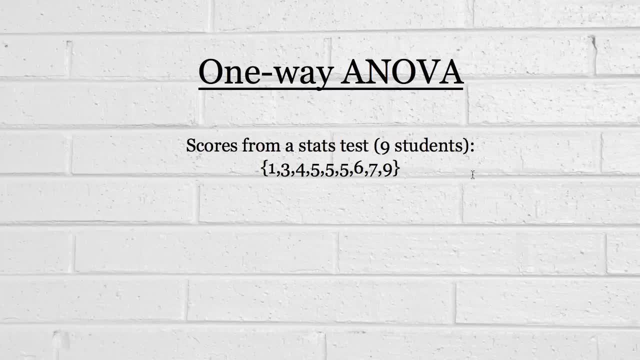 at what one way anova actually is. we're going to use this example now, which is a theoretical stats test, where there were nine students and you can see the top score was nine, perhaps out of ten, and the bottom score was one, and there was lots of scores in between. um, the first step is always: 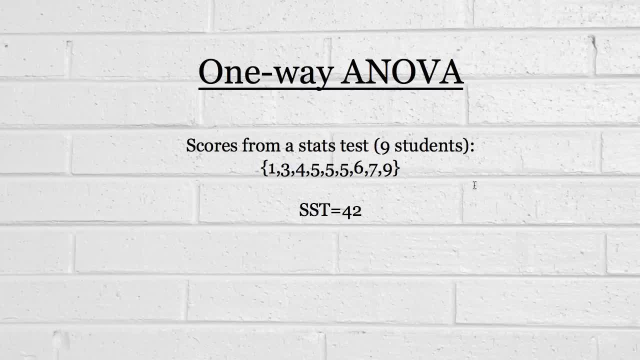 to calculate this total sum of squares. that is the variance, that's the variation i should say that we're actually dealing with, which we're going to try to explain, and the total sum of squares in this case is 42, which you can try yourself, but perhaps you'll just believe me. now, let's presume. 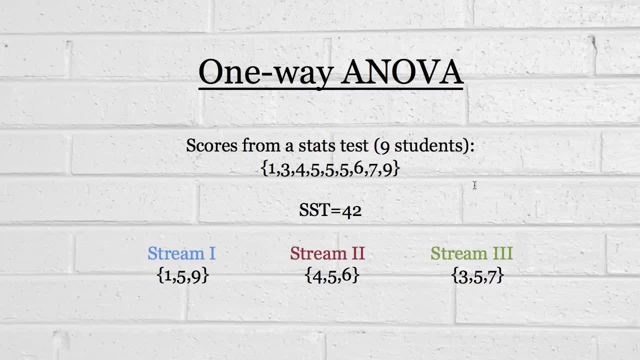 that there were three different streams or classes and you can see that in one stream we had the person that scored one, the person that scored five and someone that scored nine. in that stream, stream two, we had a four, five, six and stream three was three, five, seven. now the question. 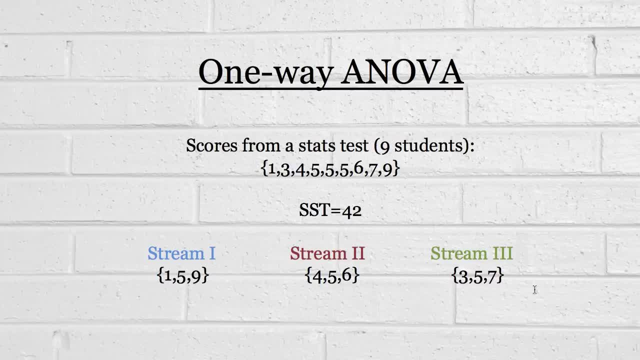 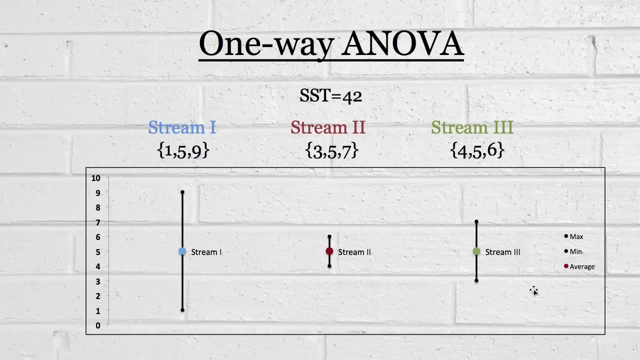 is, and this is what one way anova asks is: is there a difference between the streams? can we say that stream one did better or worse than stream two or stream three, etc. so how do we do it? here's a little plot to show you how to do it. so here's a little plot to show you how to do it. so here's a little. 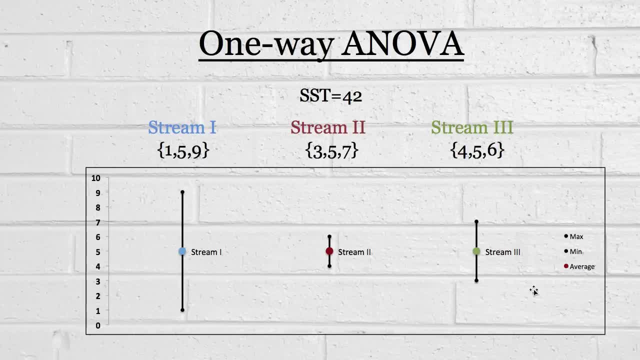 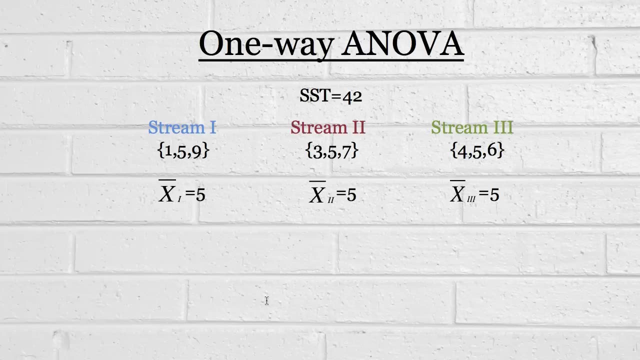 show you the three streams and i basically just put the means. they're the dots in the middle and then the maximum and minimum at the top and bottom. you can see here that the mean of each stream is actually very similar. in fact it's exactly the same. the mean of stream one is five. the mean of 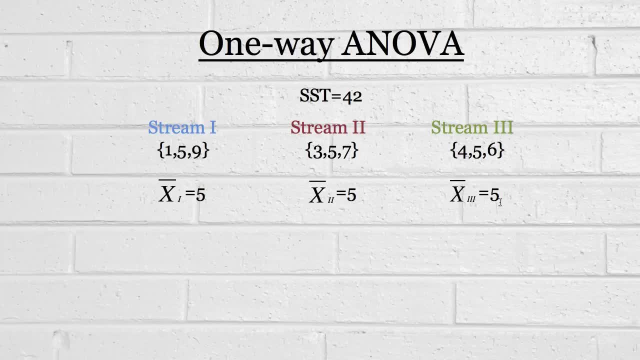 stream two is five and three is also five. so if you were asked the question- is there a difference between the three streams? you could probably say no straight away. you could probably say no away, In fact, you could definitely say no straight away. So let's just see how one-way 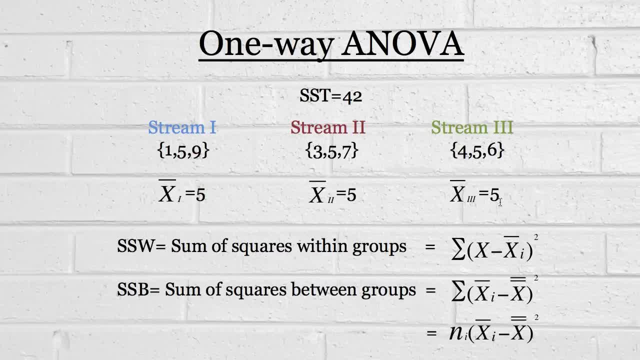 ANOVA goes about answering that question. What it does is it splits that total sum of squares into two components, which is the sum of squares within groups and the sum of squares between groups. Now they've got slightly different formulae, but I'm not going to really deal. 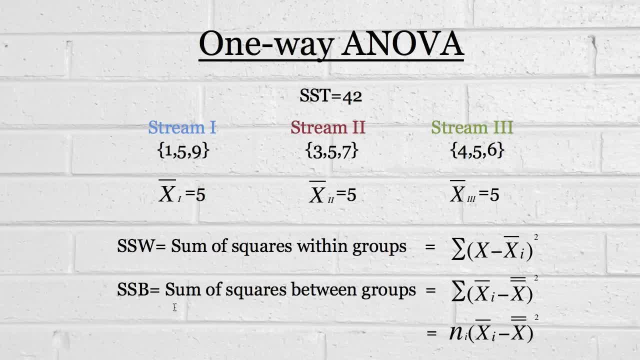 with the formulae because I feel like they're just really simple once you actually go through an example. So there they are. there You can have a look. if you're one of those people that like using formulae- I'm not, I like just running through an example and it sort of solidifies for 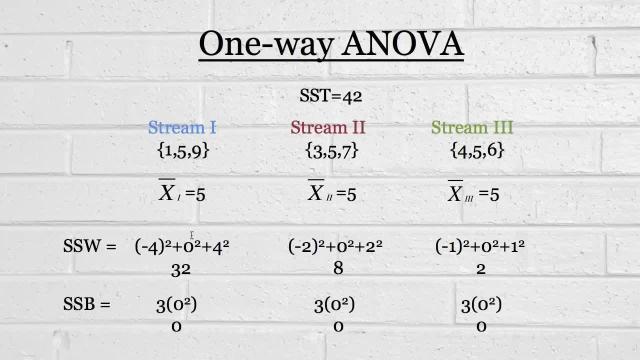 me. So let's do that. The sum of squares within groups basically focuses on the individual streams themselves. So, stream one, we have one, five and nine. The sum of squares within that group implies that we need to find the mean of that group, which is five, where we subtract five. 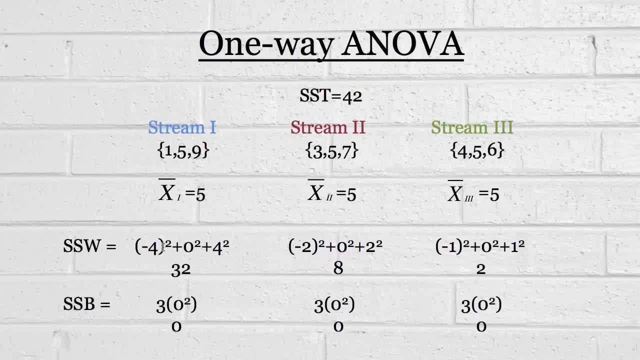 from n of the observations. So 1 minus 5 is minus 4 squared, 5 minus 5 is 0 and we square it. 9 minus 5 is 4 and we square it. So the component of the sum of 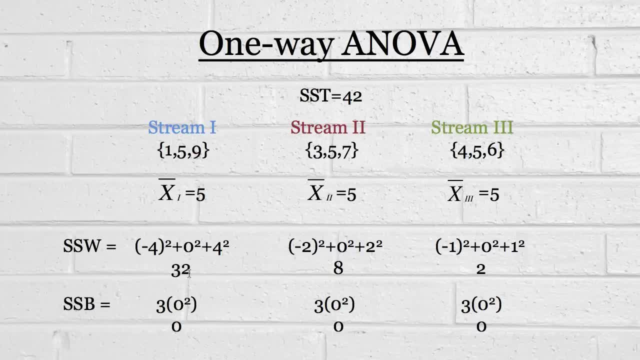 squares within groups for this particular stream is 32.. And we can do that again with stream 2, the mean of that stream is 5, we go 3 minus 5 and we get minus 2 and we square it, etc. So the total, the sum of squares within groups. 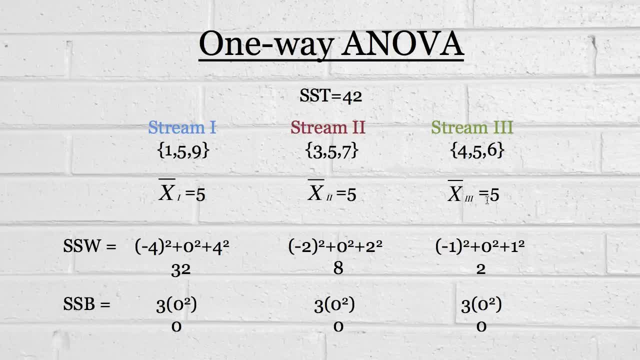 looks at the mean of the group or the mean of the stream and does that calculation, that sum of squares, calculation with that mean To find the sum of squares between groups. we're comparing the group's mean with the global mean. So here's the group mean: 5.. As it turns out, the global mean is also: 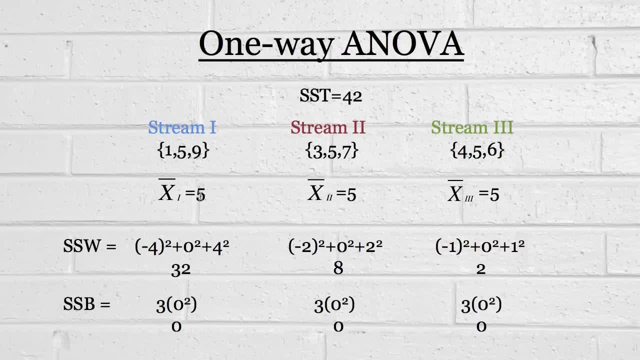 5. So what we're going to do is we're going to take five minus the global mean, five square it, but then we actually multiply it by the number of observations in the stream. That seems a bit strange, but just imagine that we're. 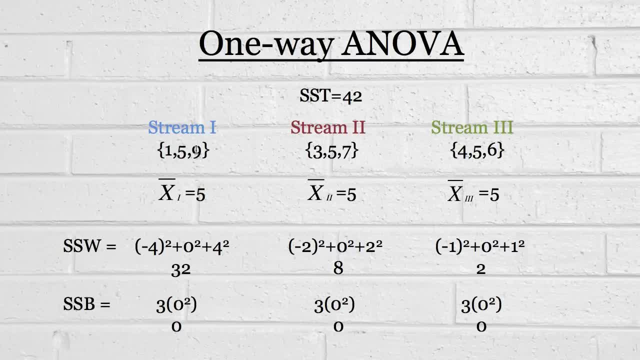 doing this calculation for each observation. So let's take the first observation. What's the mean of the group Five? What's the global mean Five? Five minus five squared is zero, And we do that with each observation, So that's why we're timesing by three in this case. In this example, though, 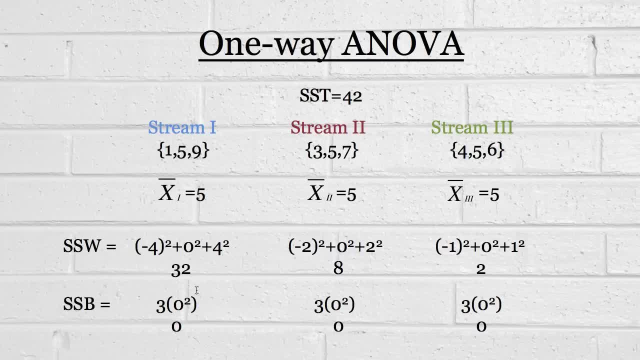 there is no between group variation. Each of these group means is equal to the global mean. So we get zero, zero, zero, And in total then we have a sum of squares within group of 42 and a sum of squares between groups of zero. So all of the variation between these nine students is 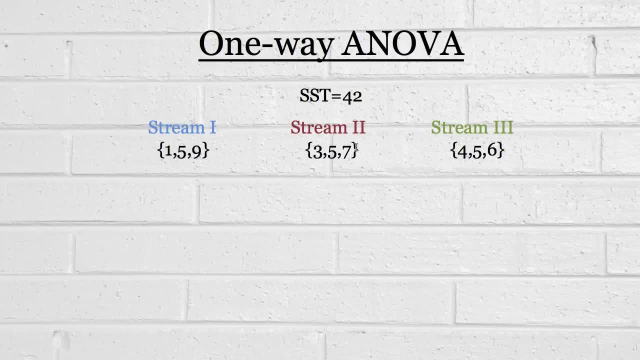 occurring within the group of zero. So we get zero, zero, zero And in total then we have a within streams. So in this next example I'm going to change the numbers around a bit. Stream one now has one, three, five, Stream two has five, seven, nine And stream three are left alone. And if we 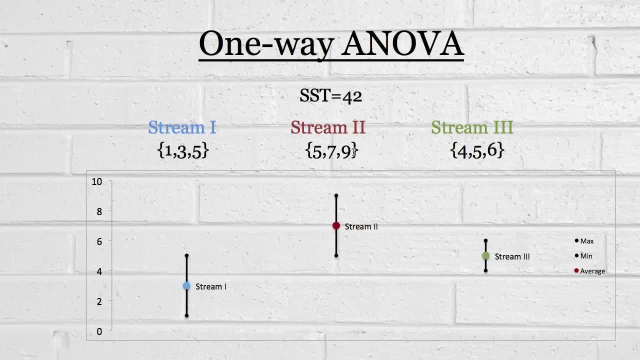 look at the plots again, you can see that there is a difference between the means. Now will one way and over tell us that that difference is significant? Again, it's possibly a good point for you to pause the video and see if you can do those calculations. So let's take a look at the 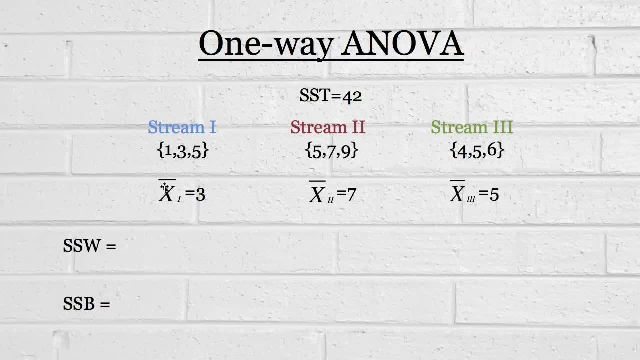 equations yourself. We've got the means of each group here: x1,, x2, and x3, the means Now finding the sum of squares within groups. I'm not going to go through it step by step, But hopefully you can. 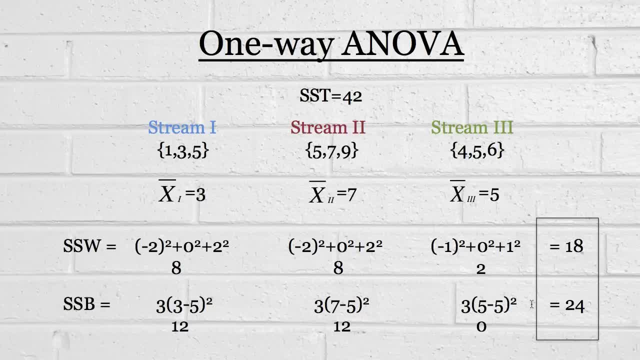 see here that the sum of squares within groups is 18 and the sum of squares between groups is 24.. So there's actually quite a decent amount of variation between the groups. So in this instance we might see that there's a statistically significant difference between the groups, And we'll see how. 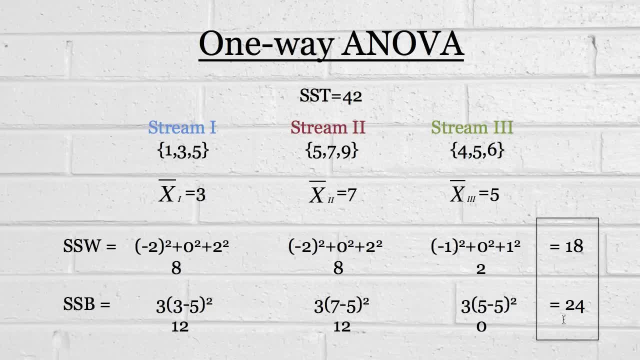 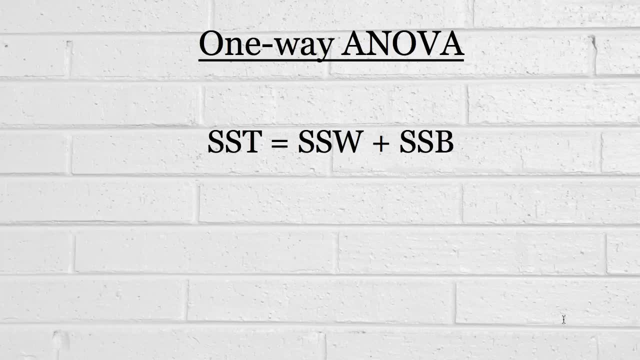 to do that in just a second. But something that becomes really evident here is that the total sum of squares is actually equal to the sum of squares within groups and the sum of squares between groups, which is actually quite an interesting property, And it's not necessarily immediately. 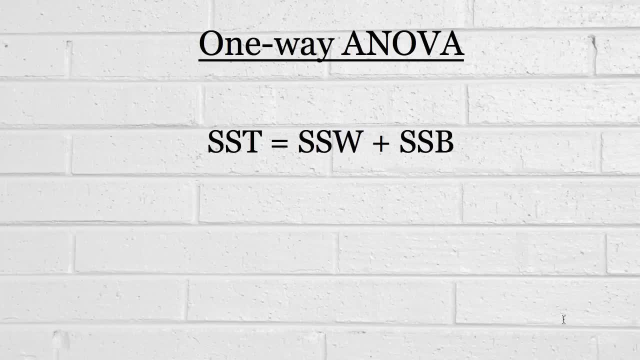 obvious why that would be the case. I'm not going to prove it here, but through the examples you might do of one way and over, you'll find that it always works out, And that's why we're going to look at that Now. as I said, we're going to need a statistical test which is going to assess. 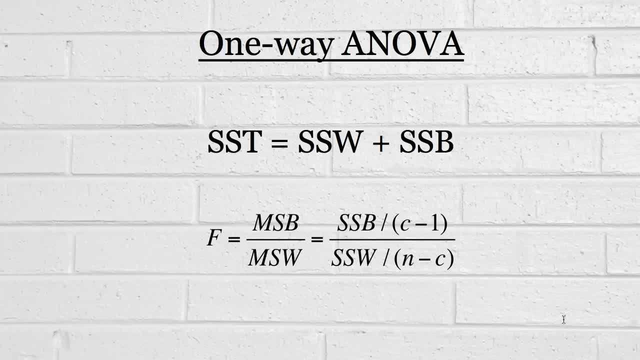 whether the sum of squares between groups is big enough to say that there's a statistical difference between the groups. means, And that's the F test, built up around this F statistic, which is the mean square between groups divided by the mean square within groups, which is just those SSB and 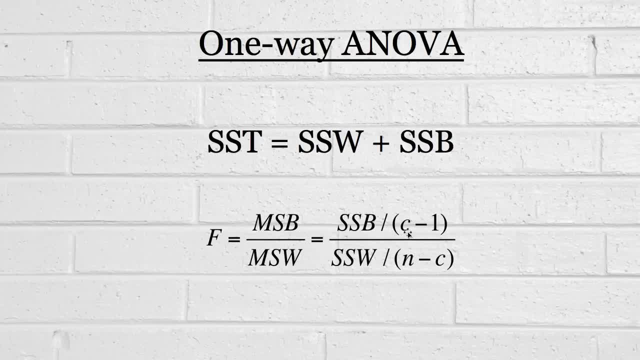 SSW figures divided by their respective degrees of freedom. I'm not going to quite go into that at the moment, but the numerator degree of freedom is just the number of categories minus one, C minus one, And the denominator is N, which was nine. That's the number of observations. 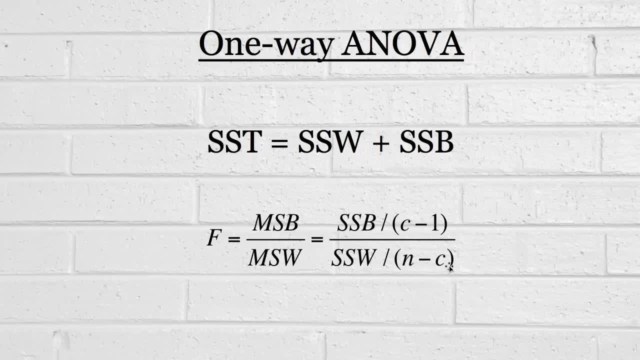 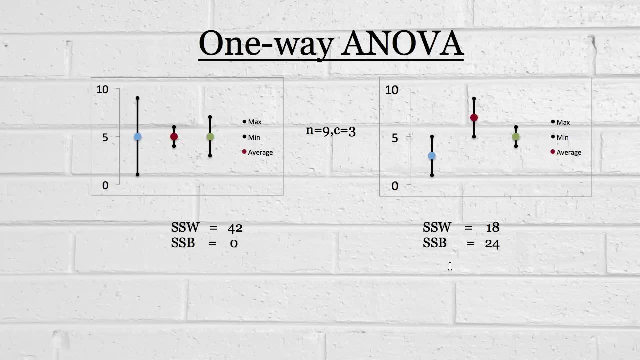 minus the number of groups. Nine minus three is going to be six. So here we have a comparison of those F statistics created for that first and second. For the second example, the first one, we had SSW 42 and SSB zero In that more recent example. 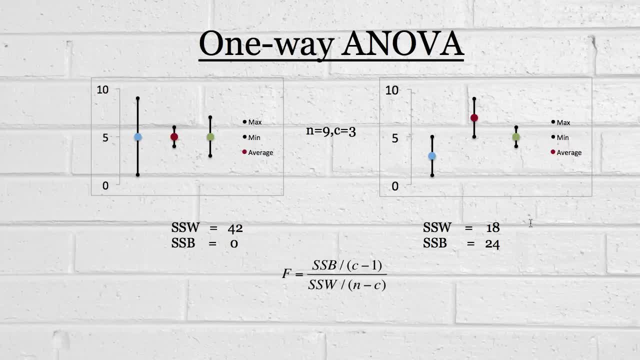 we had 18 and 24.. So if we use that calculation for F, we get an F statistic of zero for the first example and an F statistic of four for the second example. As the means get further apart from each other, our F statistic is going to increase. So if they're even further apart, 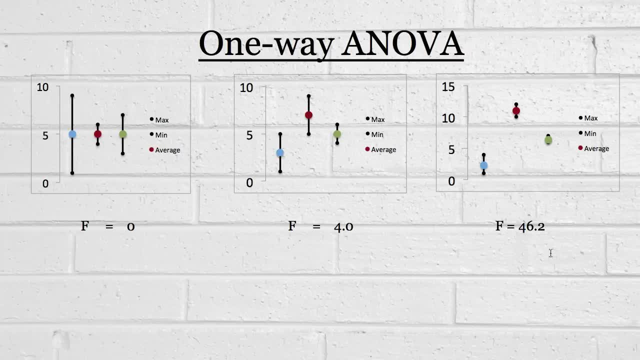 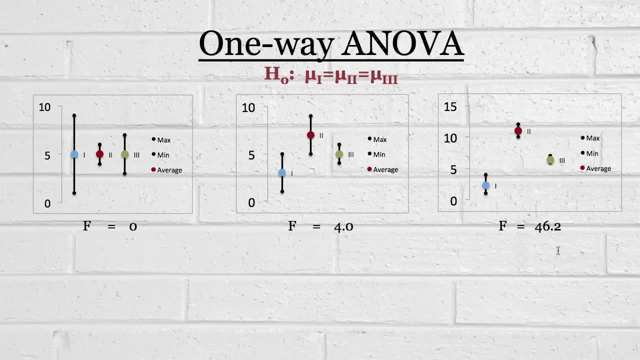 we're going to get a higher F In the previous example. we're going to get an even higher F statistic. So the actual hypothesis that these statistics are testing is whether all three means are the same, And the higher the F statistic is, the more likely we are to reject that null hypothesis. 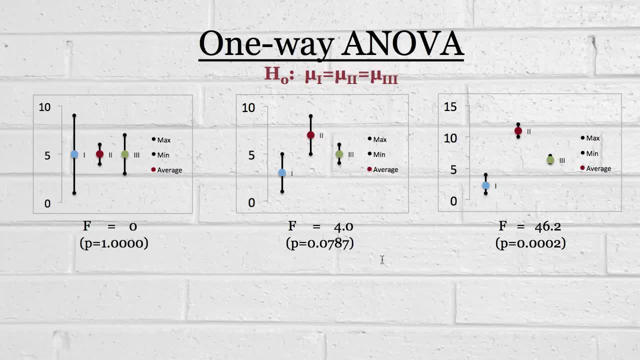 So here are the P values associated with each of the F statistics. Of course, the lower the P value, the more likely we are to reject. So using those p-values we'd say certainly in this example on the right, we'd reject H nought. 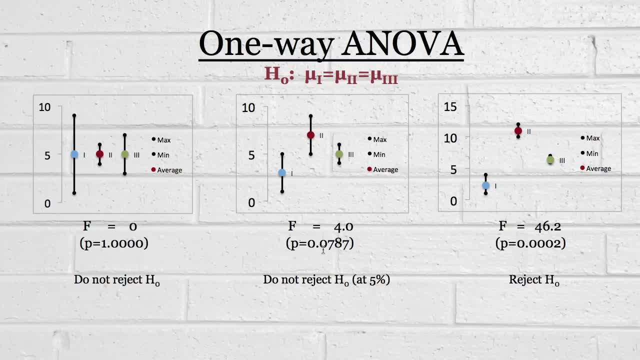 that p-value is very, very small indeed In the middle. that p-value is not quite low enough to reject this null hypothesis at the 5% level of significance, but it would at the 10% And of course, in this first example.